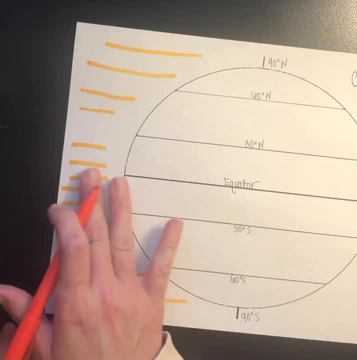 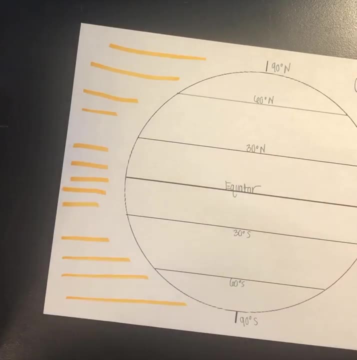 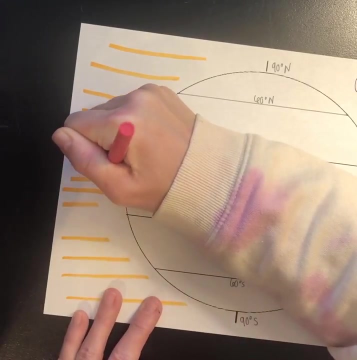 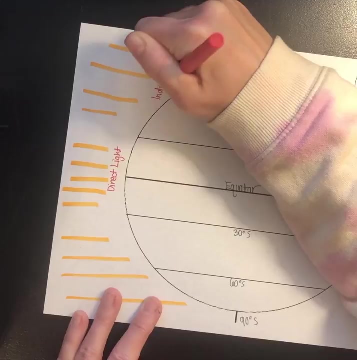 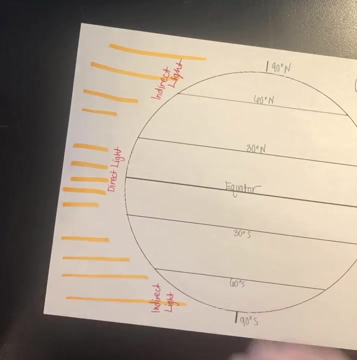 The sun lines up pretty close to our equator And as it hits the north and south pole, this curvature causes that sunlight to hit indirectly. So I'm going to label that for you guys. This is direct sunlight and indirect light, Because the sunlight's shining straight at the equator. it's going to be quite warm there. 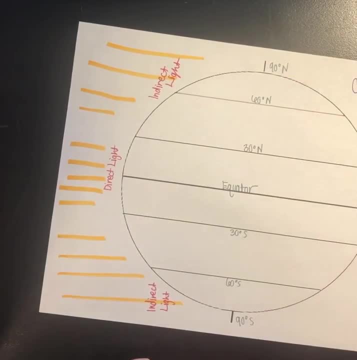 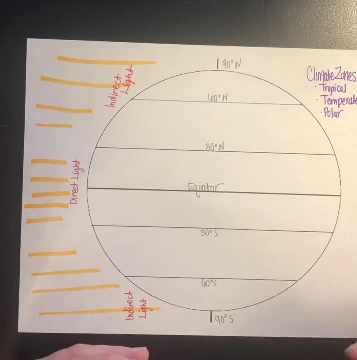 whereas the north and the south pole are going to be much, much colder. That causes our three climate zones. It also causes it's one of the factors for our weather, why we have weather across our planet. So now let's get into our climate zones. 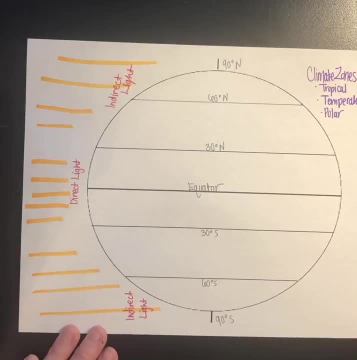 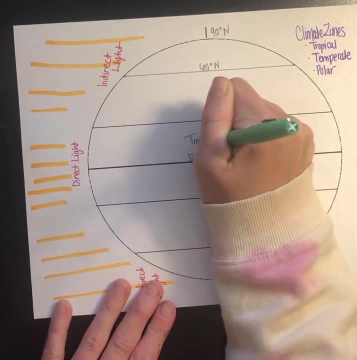 So the first one is between 30 degrees south and 30 degrees north. I'm going to use green for this one. since there's lots of rain foresting, I'm going to use red for a little bit of the weather here. This is our tropical climate zone. 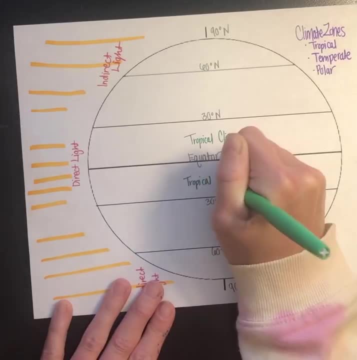 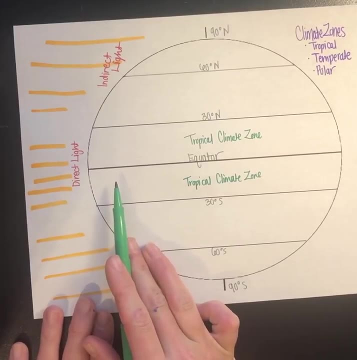 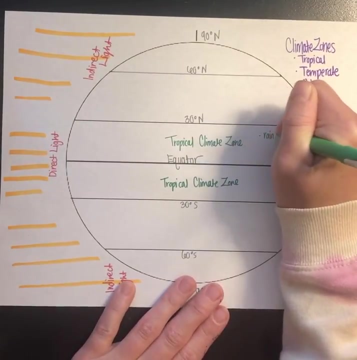 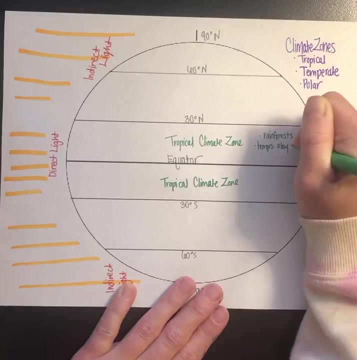 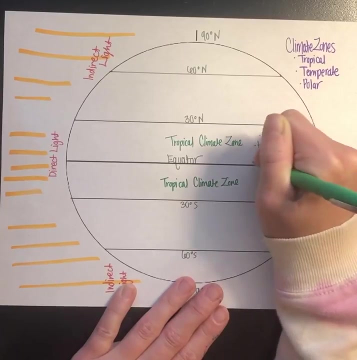 And I'm going to write it twice so that you can see the pattern. The direct sunlight coming in causes the water here to evaporate and then fall as rain. So in this climate zone we have lots and lots of rain. forests stay relatively constant throughout the year: there is a wet season and a dry season in most. 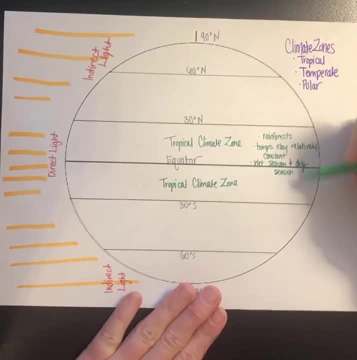 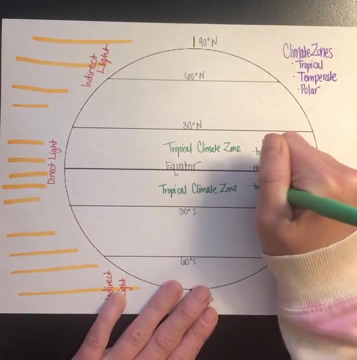 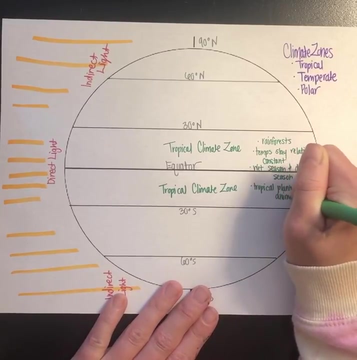 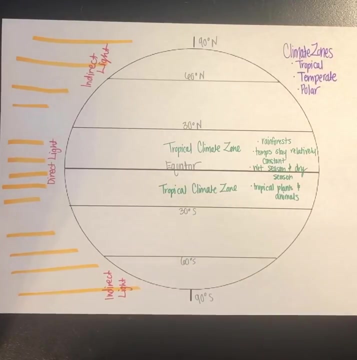 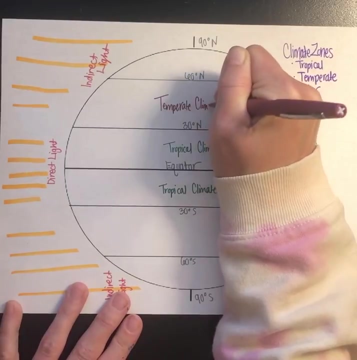 places here, but even within those seasons, the temperature is pretty constant throughout the whole year. you're going to find lots of tropical plants and animals here. the next climate zone that I'm going to talk about is our temperate climate zone. the temperate climate zone is found. 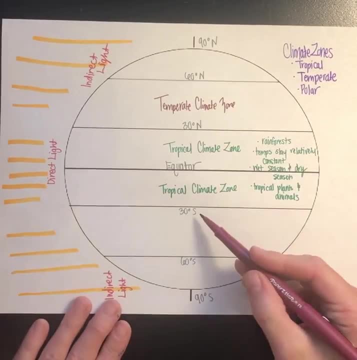 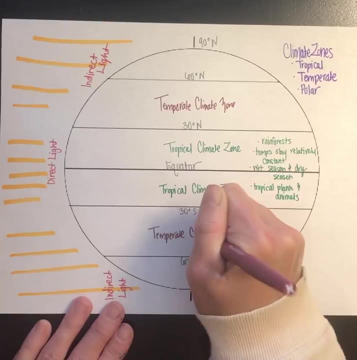 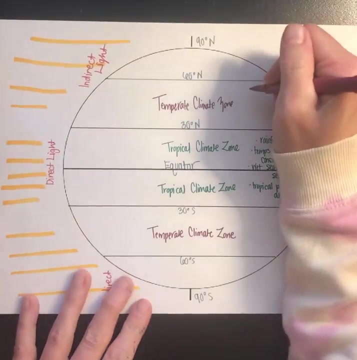 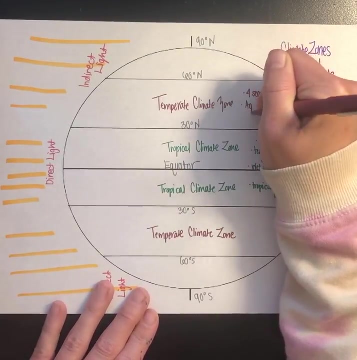 between 30 degrees north and 60 degrees north, also 30 degrees south and 60 degrees south in the temperate climate zone. you're going to get four seasons. most of Earth's agriculture, our agriculture, is found within the temperate temperate climate zone and most 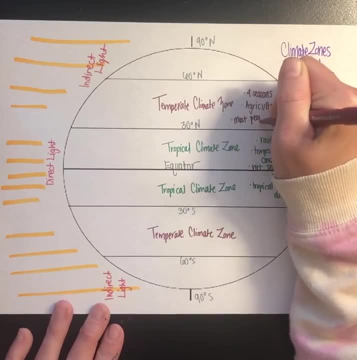 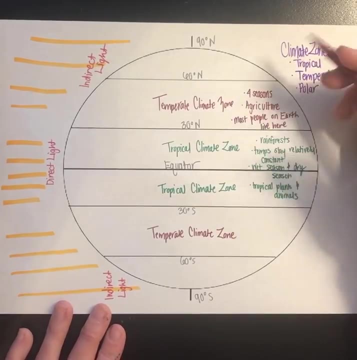 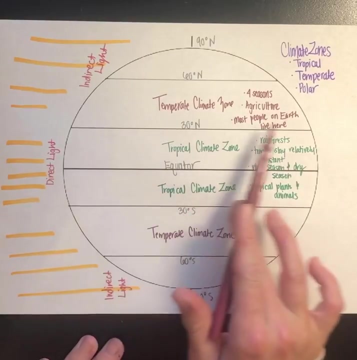 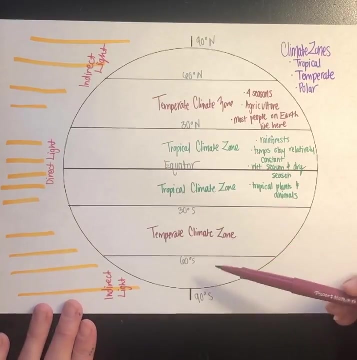 our population of people live here. There's a lot of land within 30 degrees north and 60 degrees north, so that's partly why most of Earth's population lives within this temperate climate zone. You're going to have similar climate between 30 degrees south and 60 degrees south, as you do between. 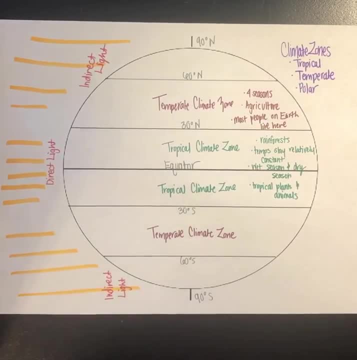 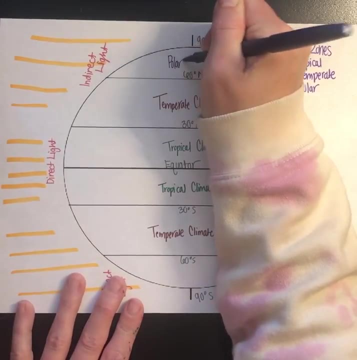 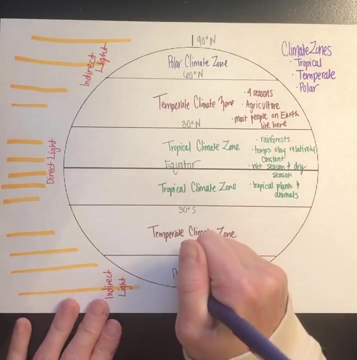 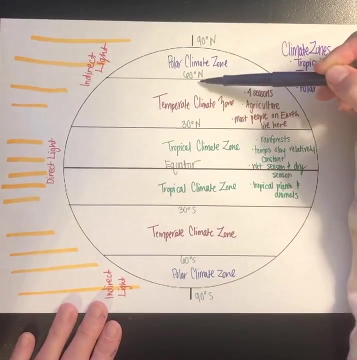 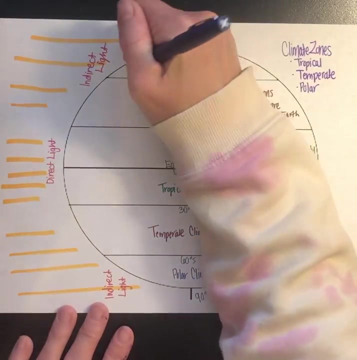 30 degrees north and 60 degrees north. The last climate zone is the polar climate zone. The polar climate zone is between 60 degrees north and 90 degrees north, 60 degrees south and 90 degrees south. That end direct sunlight causes it to be very cold there. It's also quite dry. 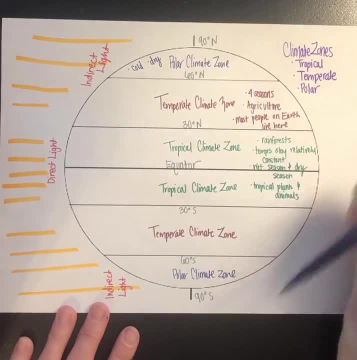 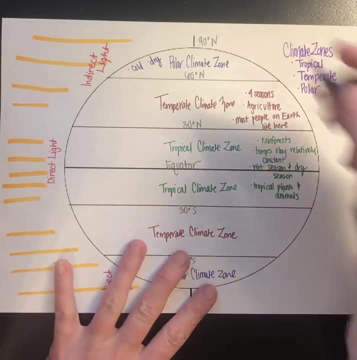 especially on the tops, like closer to the North Pole and closest to the South Pole. Most of that is ice, not snow. that you see as the white part on the map. You're going to get two seasons here. The two seasons are going to be a daytime. 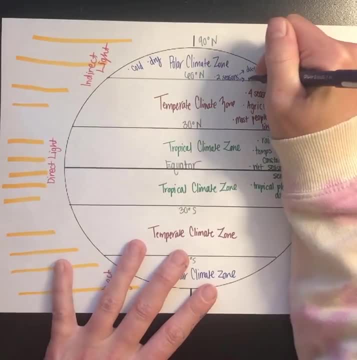 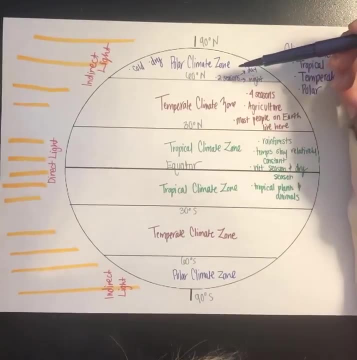 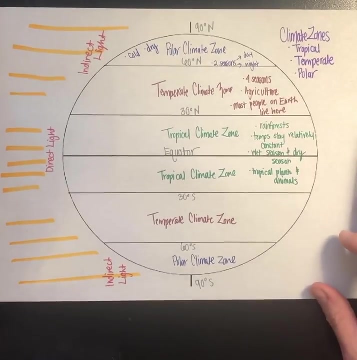 six months of daytime and six months of night. The Earth orbits the Sun at a 23.5 degree tilt. Because of that, the North Pole experiences six months of daytime and then six months of nighttime. The southern hemisphere, the South Pole, is going to experience the opposite. so when the North Pole is in 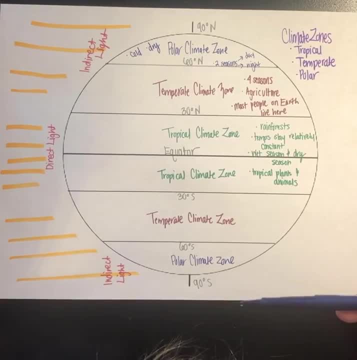 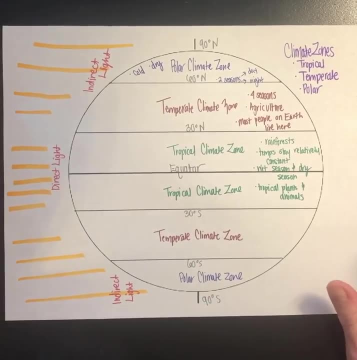 daytime or daylight. the Polar climate zone in the South Pole is going to be in six months of dark, So their seasonal change is very drastic, Going from a very long while in daytime, where the Sun doesn't set, to extreme periods of dark, where it's extremely cold.